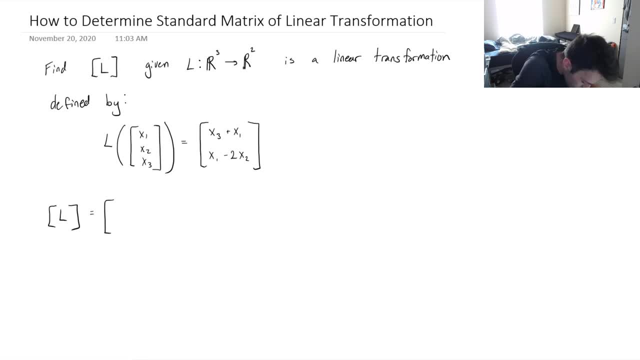 will be three columns right here, and each column being the transformed version of each of our basis vectors of R3.. So all we have to do, actually, is just calculate what these things are. So we know that E1,. 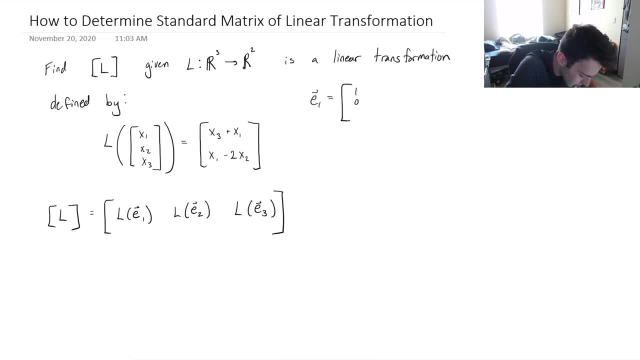 is equal to 1, 0, 0,. right, because this is a basis for R3.. So if I were to apply the linear transformation to this vector, it maps to R2, and the first component of our transformed is x3 plus x1.. 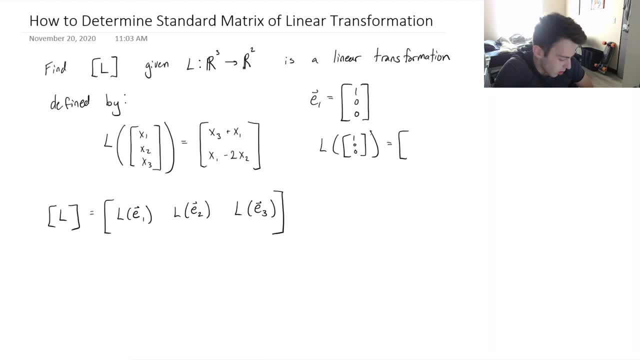 And my x3 for E1 is 0, my x1 is 1, so this is 0 plus 1, which is 1.. My second component is, similarly: it's x1 minus 2x2,, which means that it will be 1 minus 0.. 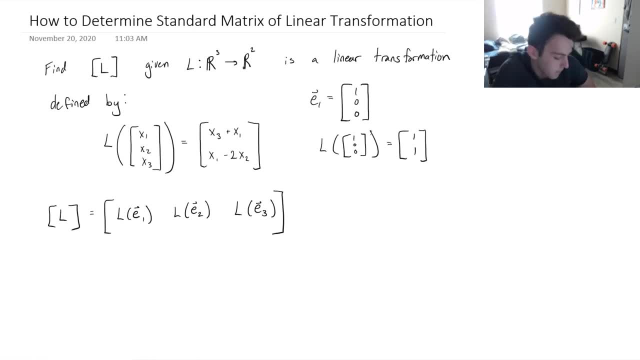 So this will map to 1, 1.. So let's take a look at E2 now. E2 would be 0, 1, 0. So applying the linear transformation to 0, 1, 0,. 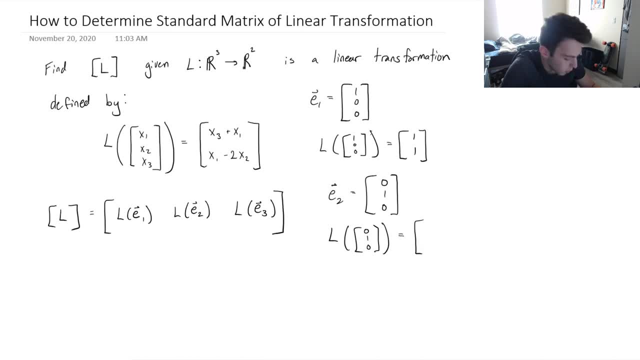 this gives us well, x3 plus x1, that's 0 plus 0. So the first component is 0. And then I've got x1 is 0 minus 2 times 1. So this will be minus 2.. 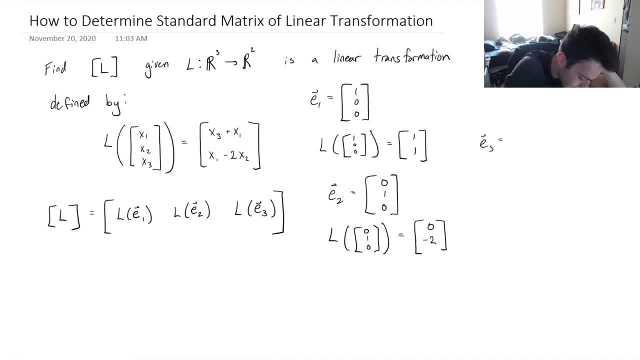 Lastly I have: E3 is equal to 0, 0, 1.. Remember, these are three components because we're starting with vectors in R3. So when I take the linear transformation of this vector, this first component is 1 plus 0, so this is 1.. 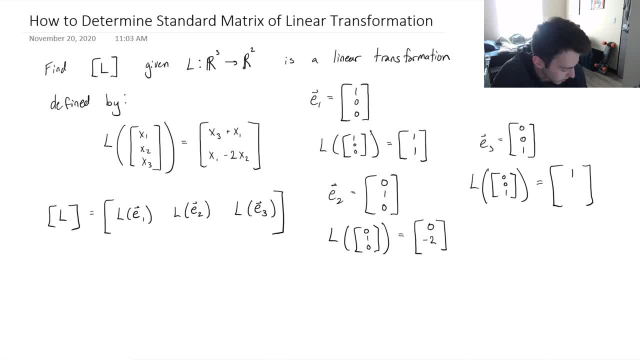 The second one is 0 minus 2 times 0 is 0. So this will be 1, 0.. So now we've got all of the columns of our standard matrix. Excuse me, So now it's as easy as just plugging them in, right? 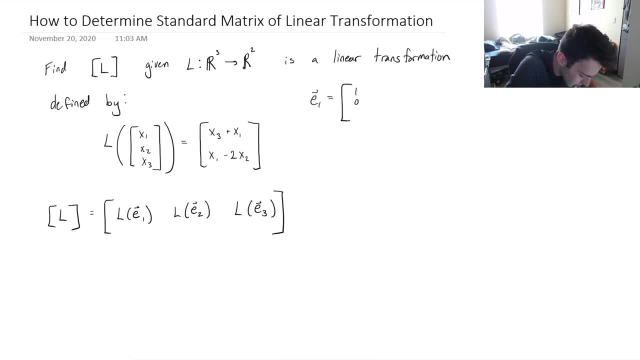 is equal to 1, 0, 0,. right, because this is a basis for R3.. So if I were to apply the linear transformation to this vector, it maps to R2, and the first component of our transformed is x3 plus x1.. 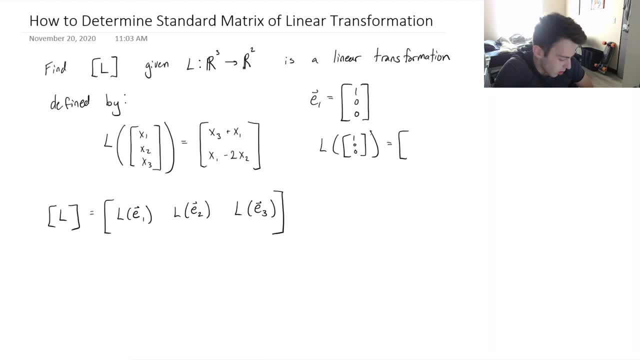 And my x3 for E1 is 0, my x1 is 1, so this is 0 plus 1, which is 1.. My second component is, similarly: it's x1 minus 2x2,, which means that it will be 1 minus 0.. 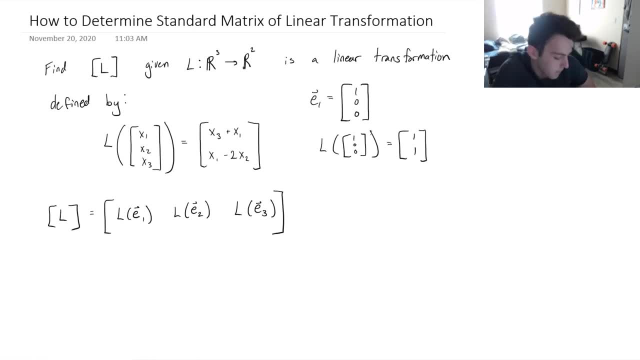 So this will map to 1, 1.. So let's take a look at E2 now. E2 would be 0, 1, 0. So applying the linear transformation to 0, 1, 0,. 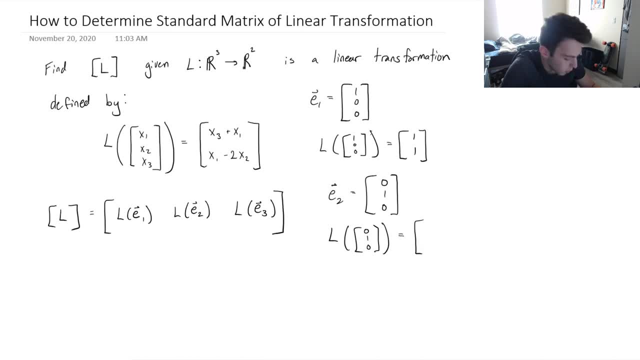 this gives us well, x3 plus x1, that's 0 plus 0. So the first component is 0. And then I've got x1 is 0 minus 2 times 1. So this will be minus 2.. 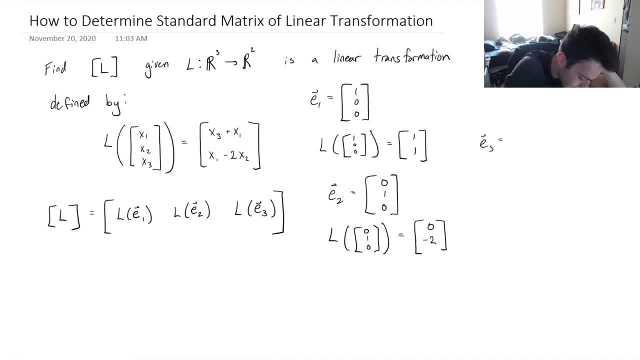 Lastly I have: E3 is equal to 0, 0, 1.. Remember, these are three components because we're starting with vectors in R3. So when I take the linear transformation of this vector, this first component is 1 plus 0, so this is 1.. 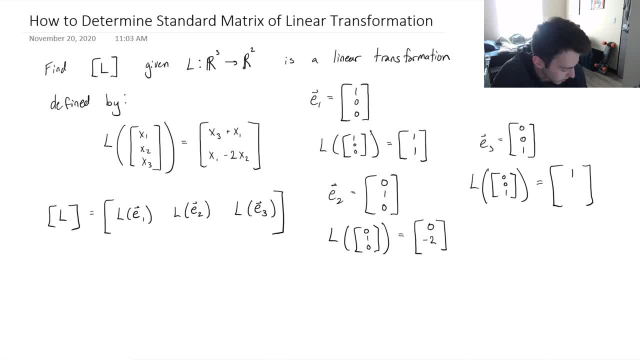 The second one is 0 minus 2 times 0 is 0. So this will be 1, 0.. So now we've got all of the columns of our standard matrix. Excuse me, So now it's as easy as just plugging them in, right? 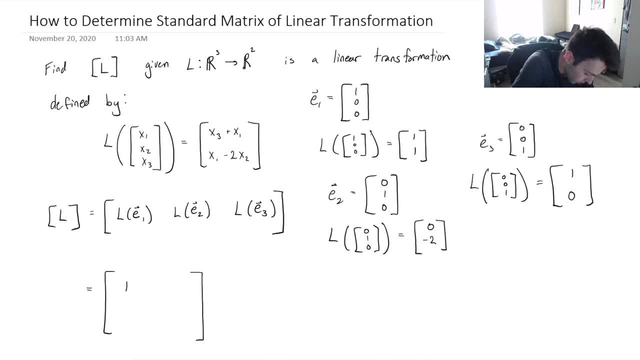 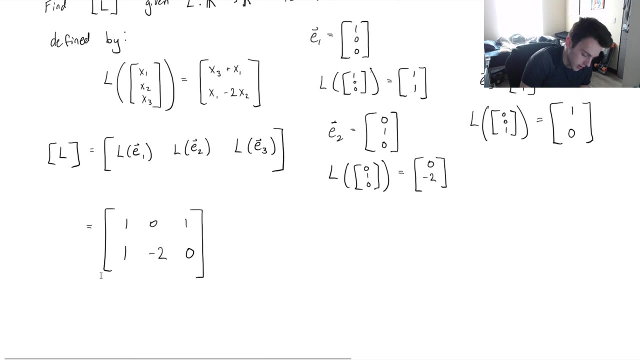 This will be 1, 1.. This will be 0, negative 2. And this will be 1, 0.. So this, right here, this is our standard matrix And this describes the linear transformation. So when I multiply this matrix by: 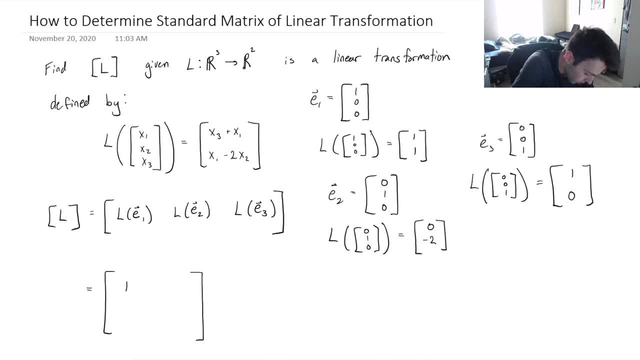 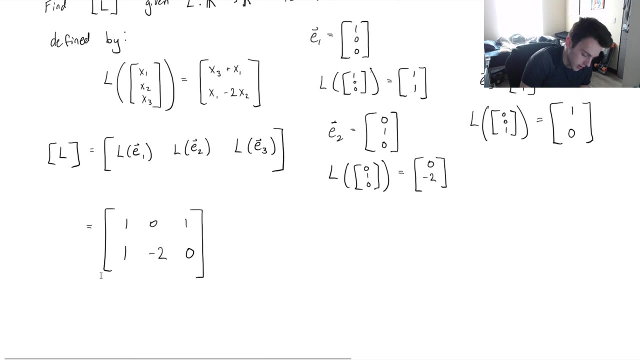 This will be 1, 1.. This will be 0, negative 2. And this will be 1, 0.. So this, right here, this is our standard matrix And this describes the linear transformation. So when I multiply this matrix by: 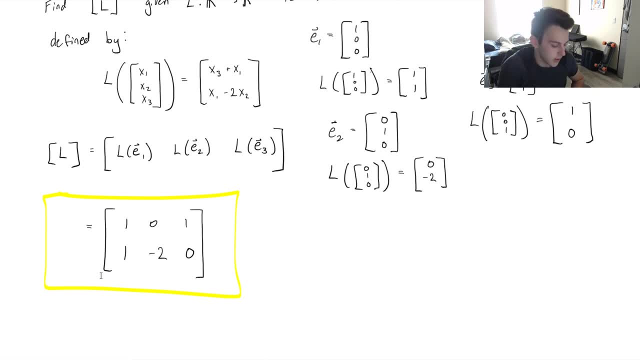 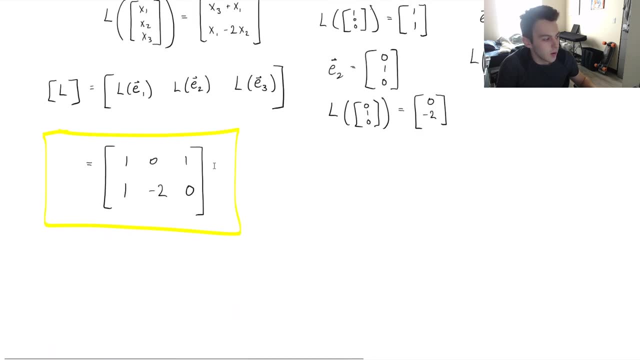 some vector right And keep in mind the vector should be in R3, because we're taking a vector from R3 to R2.. Then when I multiply it by this, this is what describes the function. It's just in terms of a matrix. now. 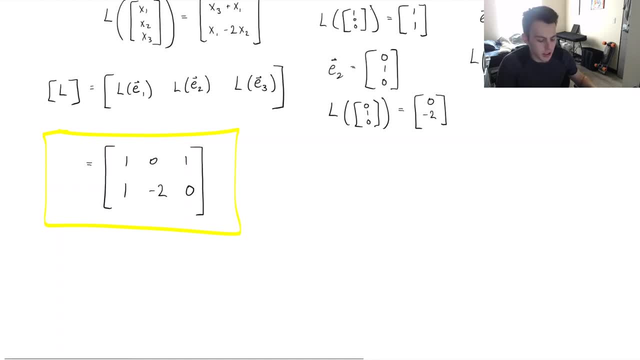 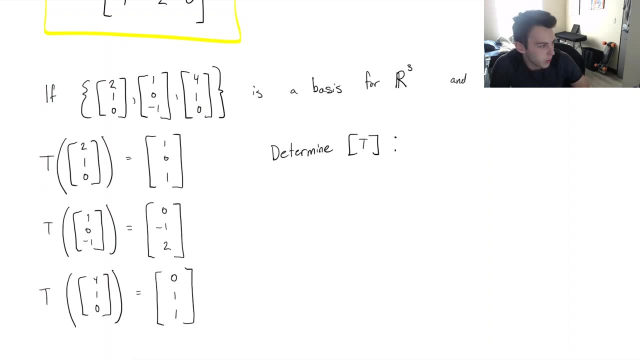 So let's look at an example where it's not as easy and the function isn't described as well for us. How can we do it in this case? So now we're given a basis for R3, and it tells us: 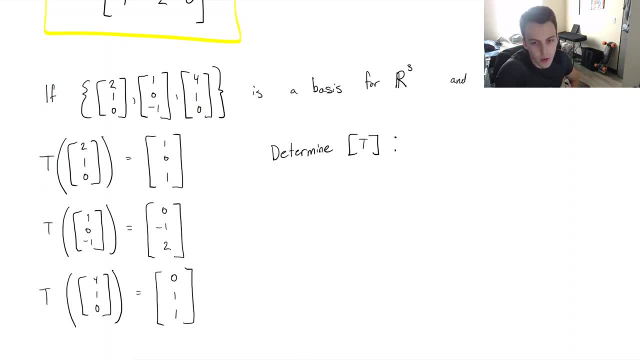 and it doesn't say explicitly here. but we can assume that T is also another linear transformation. But this time it takes a vector in R3, and it spits out another vector in R3. And we know where each of our basis vectors for R3,. 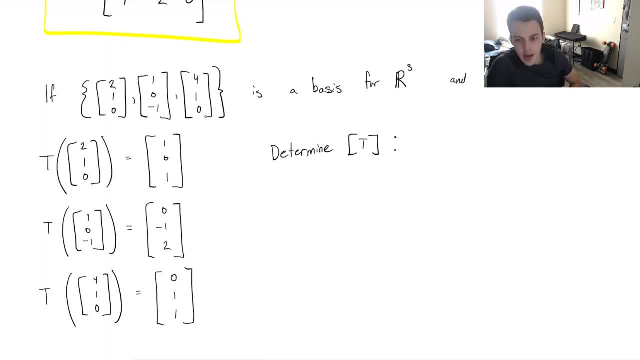 are output to, But they're not the standard basis vectors. So how could we find the standard matrix T in this case? And the important thing to notice here is that, since the vectors that we were given, it tells us that this is a basis for R3.. 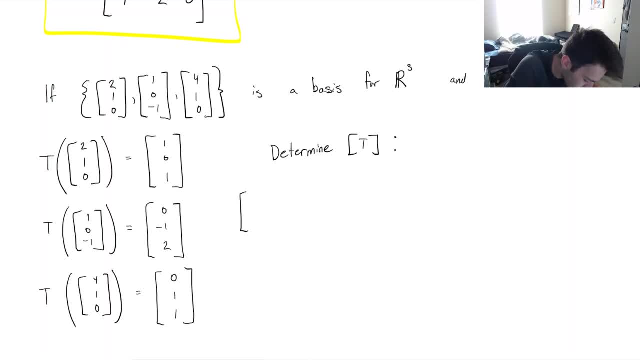 It means that we can express any vector in R3 as a linear combination of those basis vectors. So I'm just going to write that out: the linear combination of those basis vectors that we've been given. Right, It's a linear combination of these basis vectors. 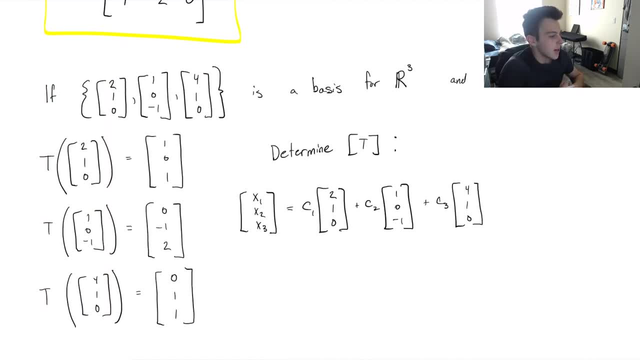 that we've been given. Since it's a basis for R3, it means that they will span all of R3. So I can come up with any vector x that is a linear. I can come up with any vector x in R3,. 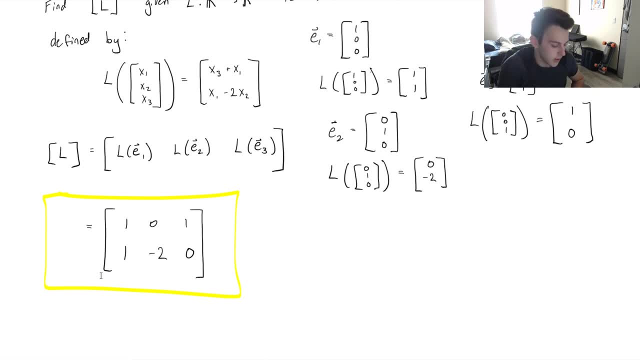 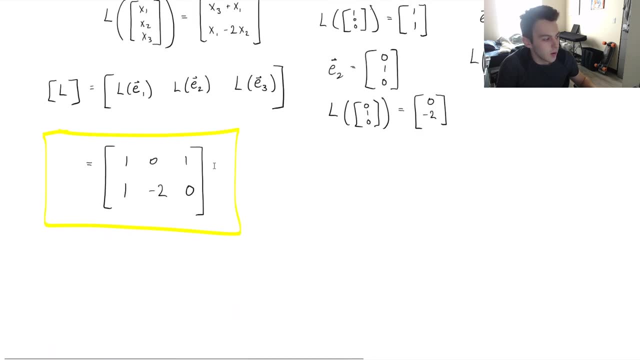 some vector right And keep in mind the vector should be in R3, because we're taking a vector from R3 to R2.. Then when I multiply it by this, this is what describes the function. It's just in terms of a matrix. now. 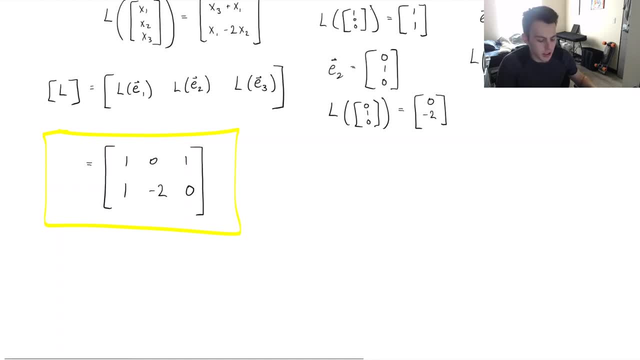 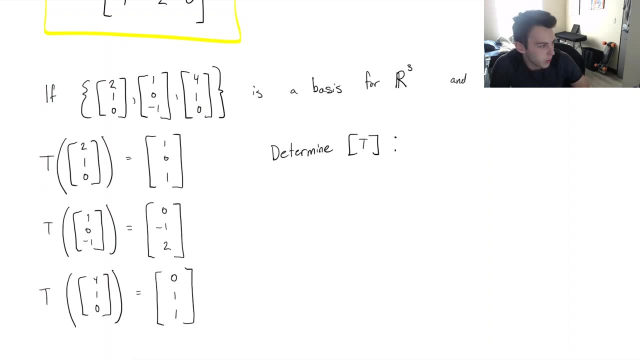 So let's look at an example where it's not as easy and the function isn't described as well for us. How can we do it in this case? So now we're given a basis for R3, and it tells us: 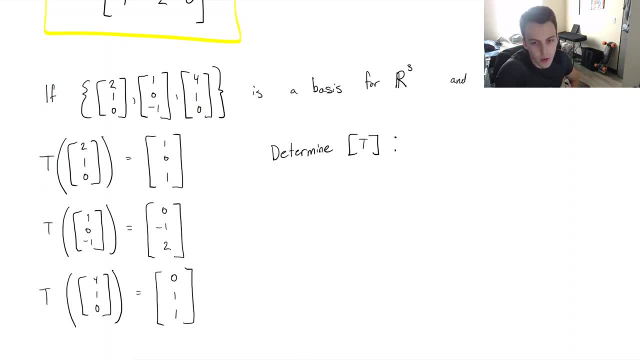 and it doesn't say explicitly here. but we can assume that T is also another linear transformation. But this time it takes a vector in R3, and it spits out another vector in R3. And we know where each of our basis vectors for R3,. 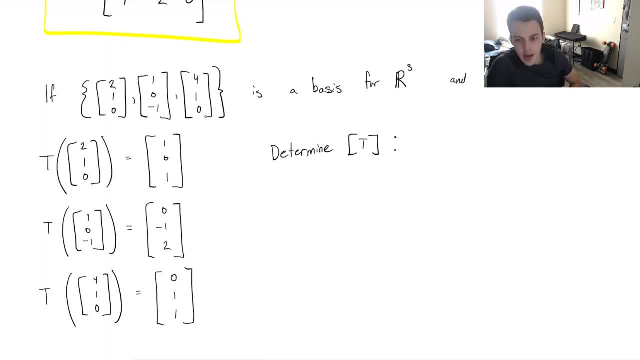 are output to, But they're not the standard basis vectors. So how could we find the standard matrix T in this case? And the important thing to notice here is that, since the vectors that we were given, it tells us that this is a basis for R3.. 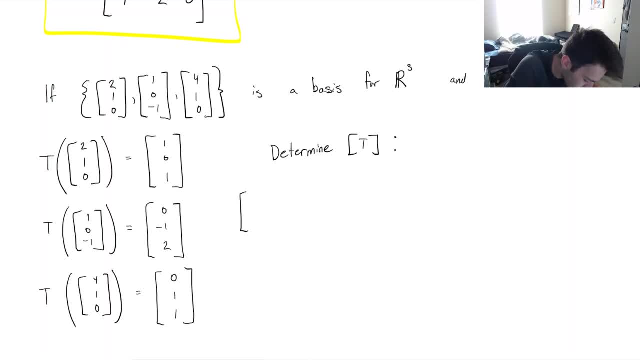 It means that we can express any vector in R3 as a linear combination of those basis vectors. So I'm just going to write that out: the linear combination of those basis vectors that we've been given. Right, It's a linear combination of these basis vectors. 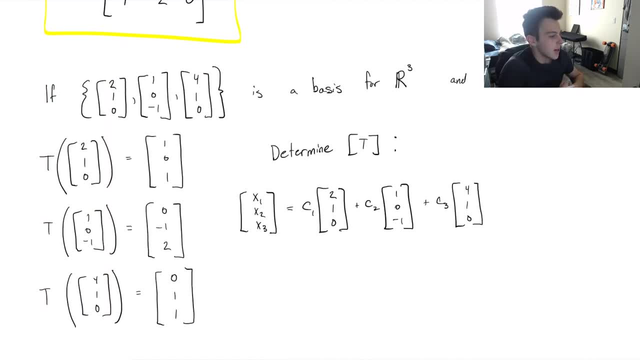 that we've been given. Since it's a basis for R3, it means that they will span all of R3. So I can come up with any vector x that is a linear. I can come up with any vector x in R3,. 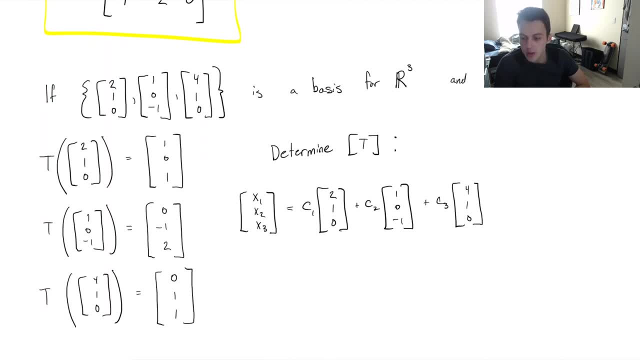 that's a linear combination of these basis vectors. So what I want to do here is actually take this into reduced rational long form and put this into a matrix. So let me just write out this matrix where I've got. 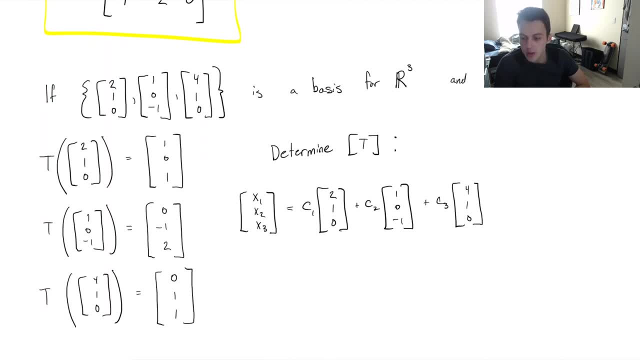 that's a linear combination of these basis vectors. So what I want to do here is actually take this into reduced rational long form and put this into a matrix. So let me just write out this matrix where I've got. 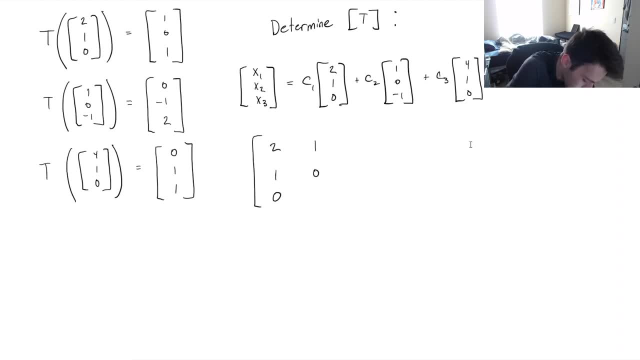 2, 1, 0, 1, 0, negative 1, 4, 1, 0, and then x1,, x2,, x3, on my other side, And what I want to do is: 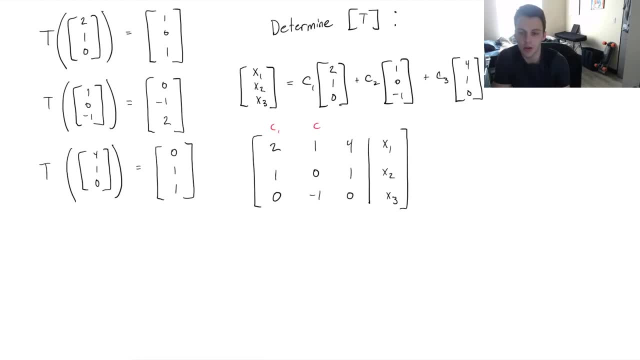 is solve for these constants Right, And it's easiest to solve for these constants in terms of a matrix, And the point of this video is not to show you how to row reduce, And there's lots of things online that can teach you this. 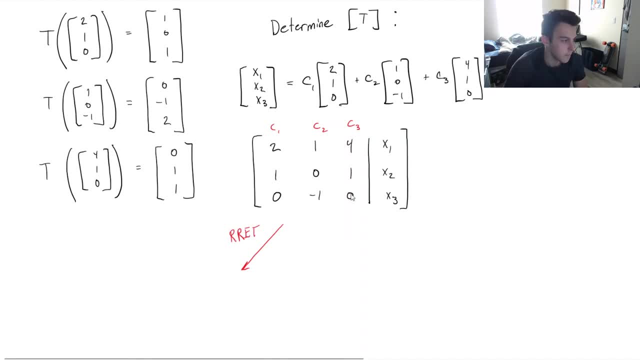 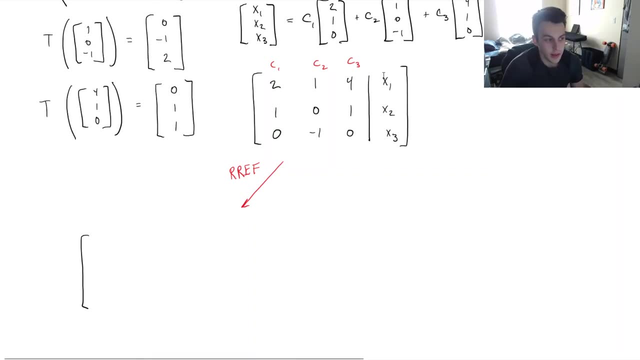 So I'm just going to skip to reduced rational long form here, And I think I actually even have a video on my channel where I do something very similar when we have like unknowns here on this, right on our augmented side. 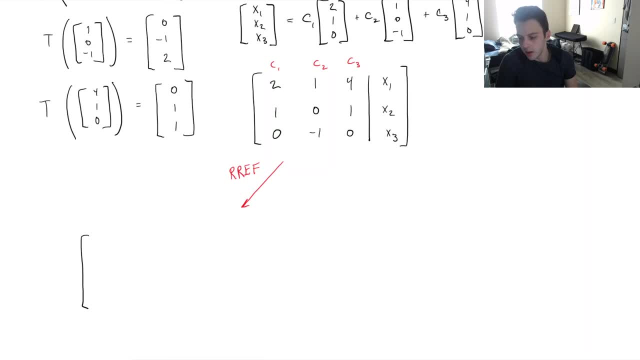 But this will result in a matrix that looks something like this: Let me just copy this down: And then we've got x3 over 2, plus 2, x2, plus x1 over 2, minus x3,. 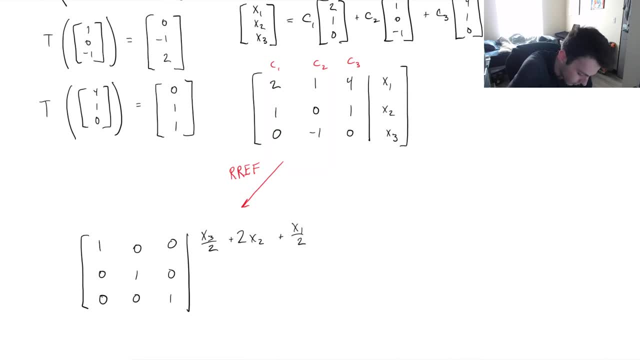 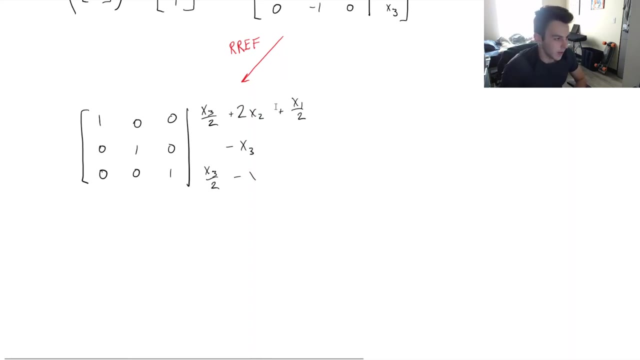 and then we've got solid. So we can see just reading the results right off of this matrix, Like if we were to look at the first row here, we can directly read off what c1 would be equal to. 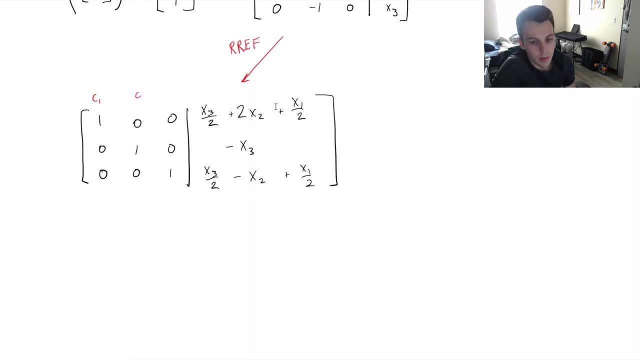 We can directly read off what c2 is equal to from the second row, And we can directly read off what c3 is equal to from the third row of this matrix. So let me just write out what this actually would look like. 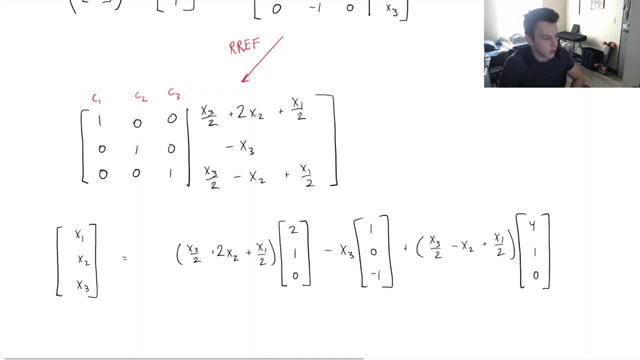 in terms of a linear combination. So putting this, putting our results from our reduced rational form back into the linear combination. it would look something like this And you might be thinking like: how is this even related? And 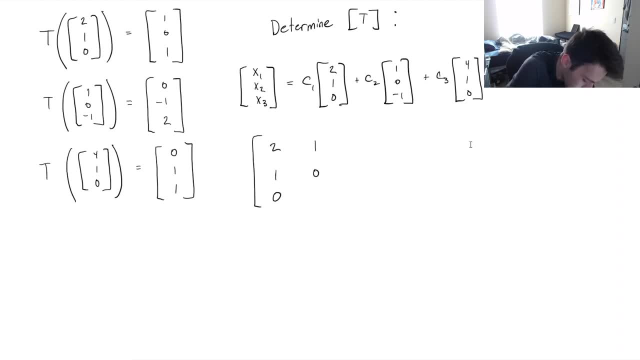 2, 1, 0, 1, 0, negative 1, 4, 1, 0, and then x1,, x2,, x3, on my other side, And what I want to do is: 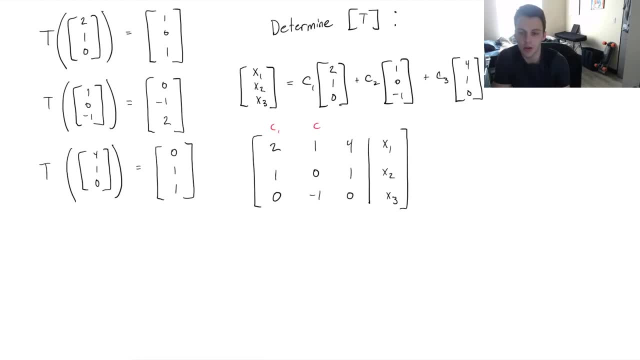 is solve for these constants Right, And it's easiest to solve for these constants in terms of a matrix, And the point of this video is not to show you how to row reduce, And there's lots of things online that can teach you this. 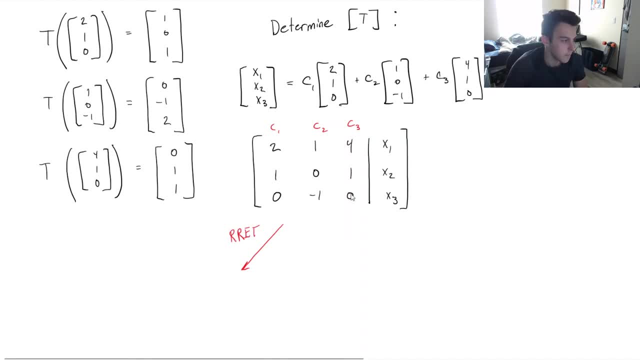 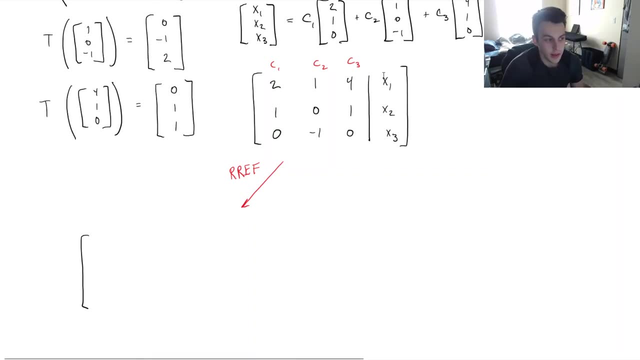 So I'm just going to skip to reduced rational long form here, And I think I actually even have a video on my channel where I do something very similar when we have like unknowns here on this, right on our augmented side. 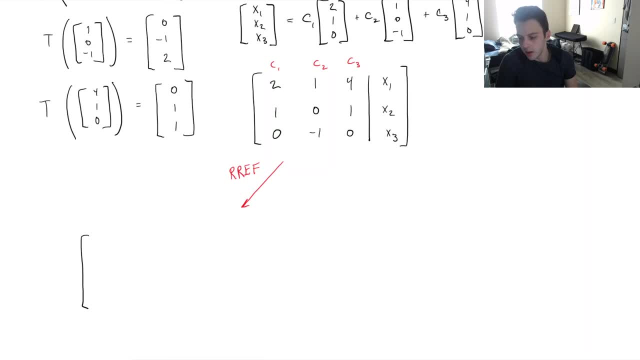 But this will result in a matrix that looks something like this: Let me just copy this down: And then we've got x3 over 2, plus 2, x2, plus x1 over 2, minus x3,. 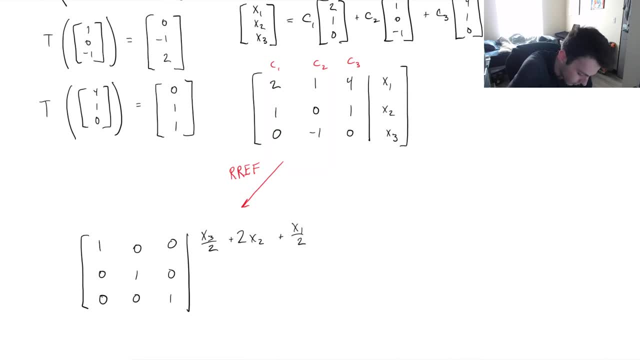 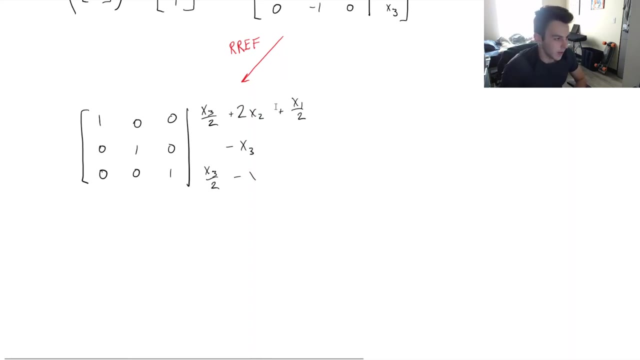 and then we've got solid. So we can see just reading the results right off of this matrix, Like if we were to look at the first row here, we can directly read off what c1 would be equal to. 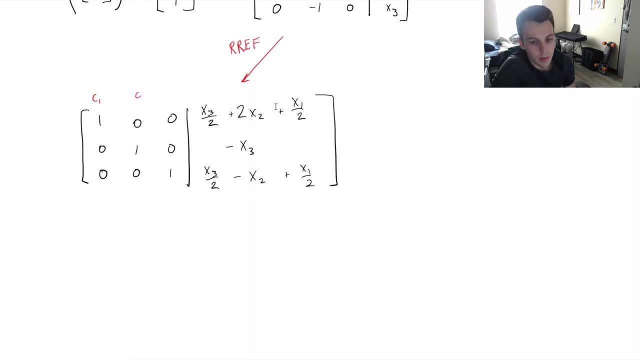 We can directly read off what c2 is equal to from the second row, And we can directly read off what c3 is equal to from the third row of this matrix. So let me just write out what this actually would look like. 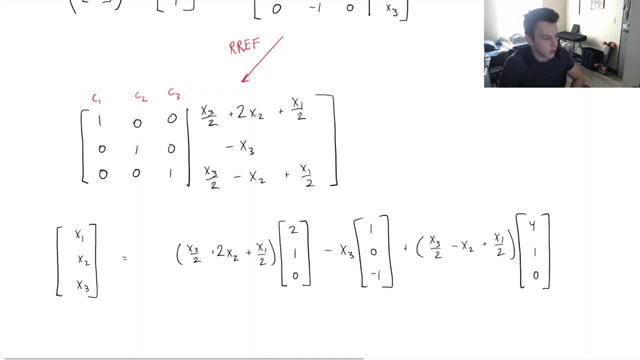 in terms of a linear combination. So putting this, putting our results from our reduced rational form back into the linear combination. it would look something like this And you might be thinking like: how is this even related? And 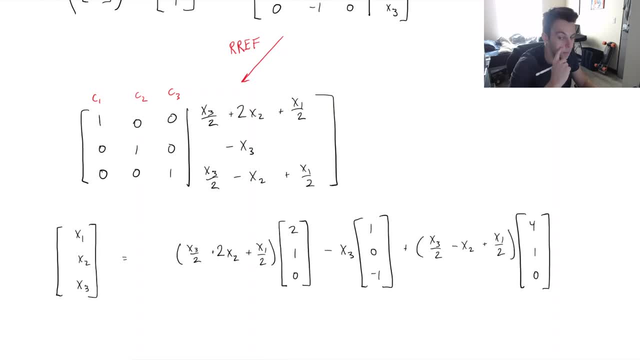 I'll show you in just a second here. If we were to take the, the linear transformation of both sides, right, The linear transformation T that's been defined for us, It would look something like this, right So: 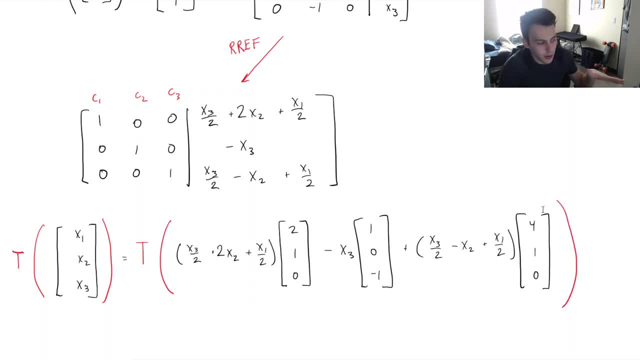 we've got T, the, the transformed, the transformed version of any vector is equal to this, this whole right hand side, And this is good because ideally we're, if we can solve for like some sort of expression. 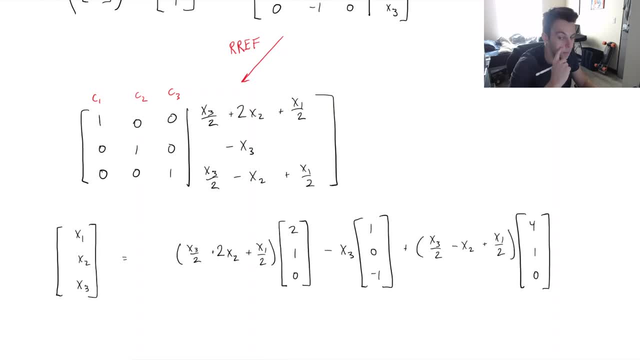 I'll show you in just a second here. If we were to take the, the linear transformation of both sides, right, The linear transformation T that's been defined for us, It would look something like this, right So: 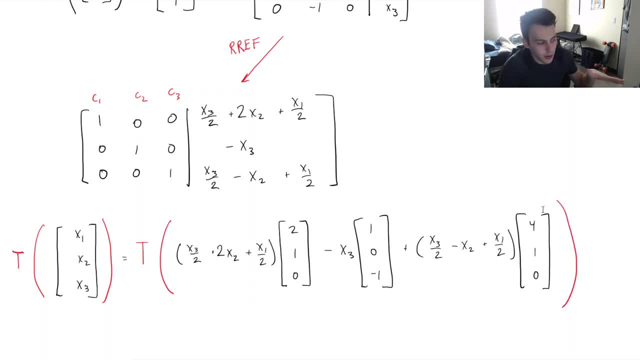 we've got T, the, the transformed, the transformed version of any vector is equal to this, this whole right hand side, And this is good because ideally we're, if we can solve for like some sort of expression. 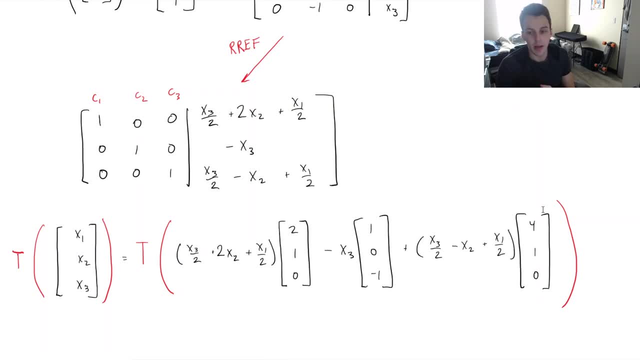 for like to describe our linear transformation. then we can break it up into a vector times a matrix, right? So really we just want to focus on the right hand side here and see what we can do. 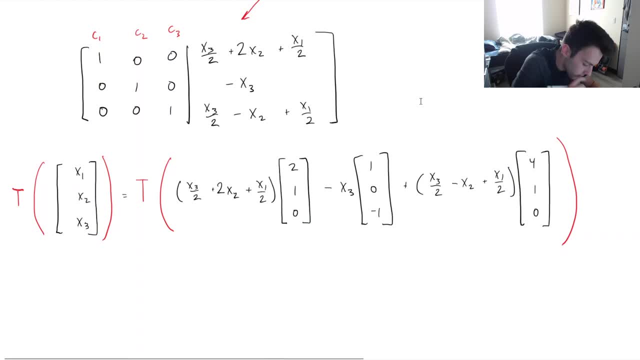 to simplify this, Right, And you might be thinking: what the heck like, how can I even simplify this? And it's important to remember that there's two, two things that we know about a linear transformation. 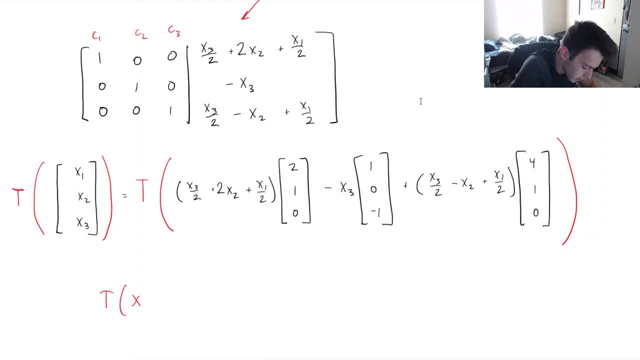 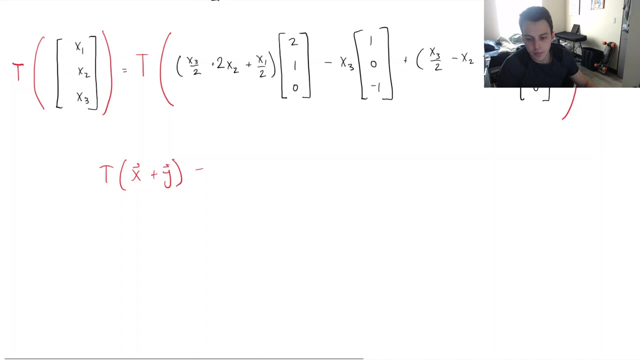 And it's when we have the addition of two vectors right that are being transformed. it's equal to the transformed version of the first vector plus the transformed version of the second vector Right. And 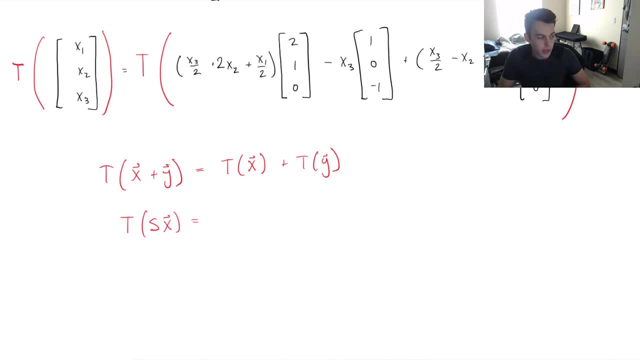 another thing that we know is that if we have a scalar times a vector and we transform that, it's equal to the scalar multiplied by the transformed version of just the vector itself. Right, And you can see here. 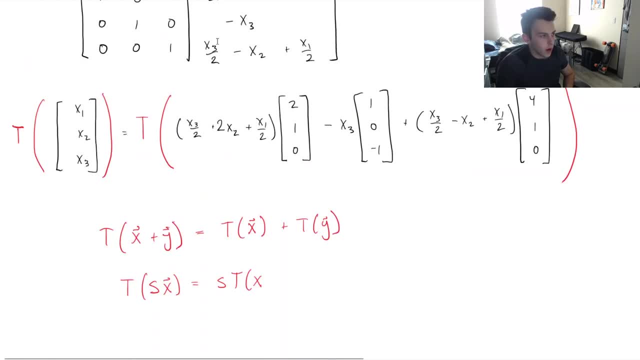 how we do have that three times Right. You've got this, this first vector multiplied by some scalar, and then we've got we're adding another vector multiplied by a scalar, and then we're adding another vector. 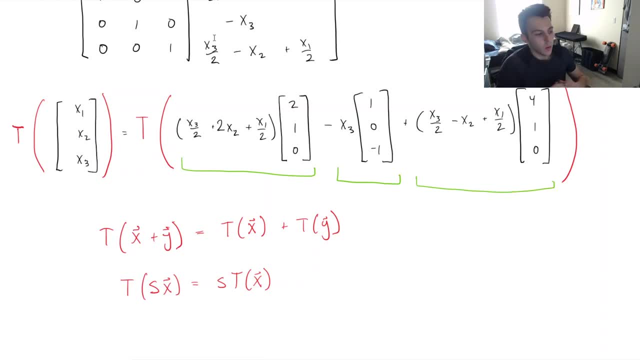 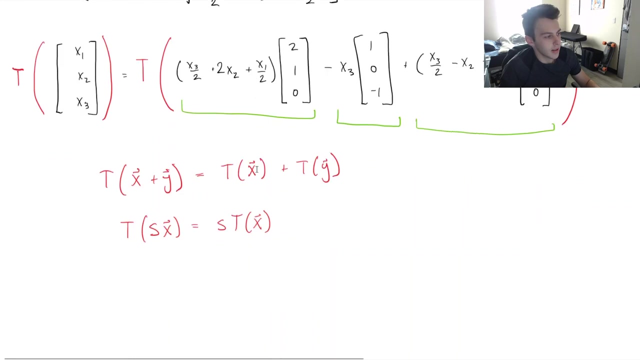 multiplied by a scalar. So what the key thing to to notice here is that linear transformations are conserved under linear combinations. So we can break this up. So let let's- let's simplify this a little bit. 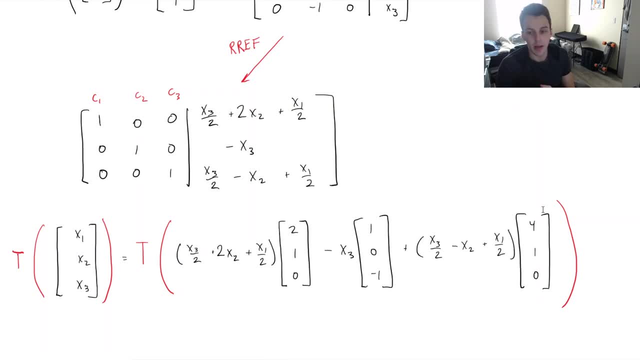 for like to describe our linear transformation. then we can break it up into a vector times a matrix, right? So really we just want to focus on the right hand side here and see what we can do. 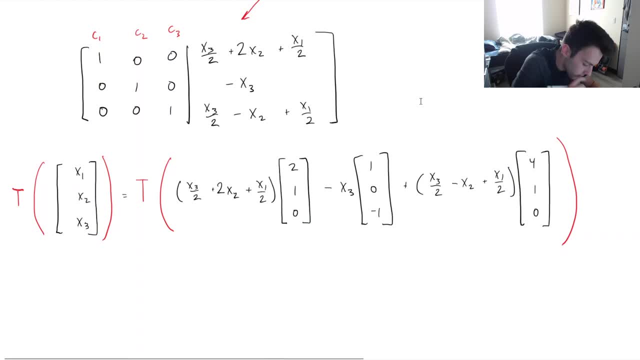 to simplify this, Right, And you might be thinking: what the heck like, how can I even simplify this? And it's important to remember that there's two, two things that we know about a linear transformation. 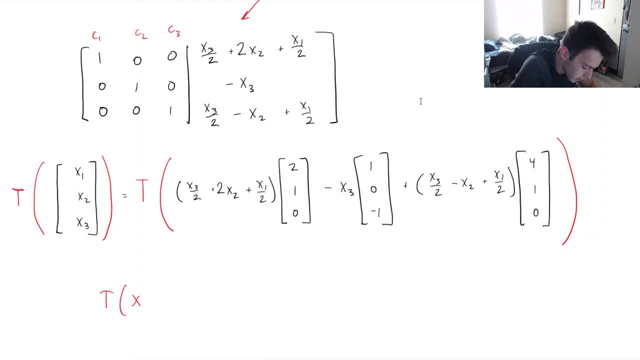 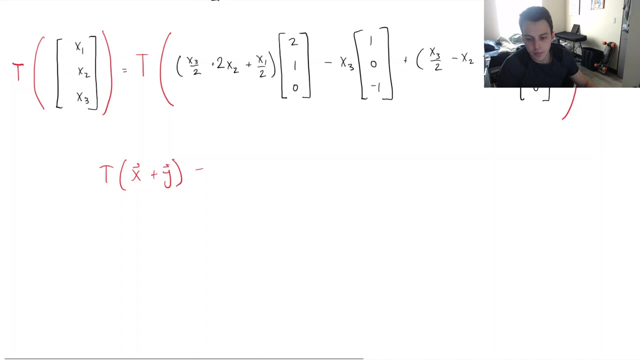 And it's when we have the addition of two vectors right that are being transformed. it's equal to the transformed version of the first vector plus the transformed version of the second vector Right. And 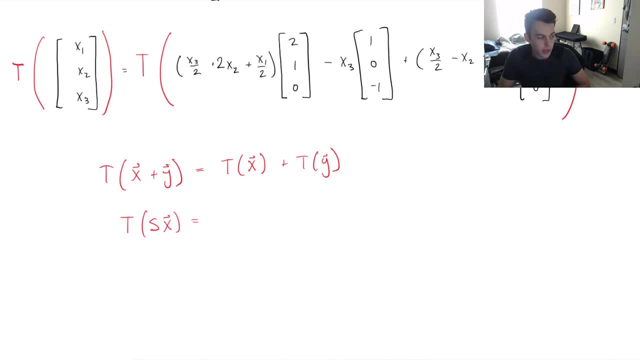 another thing that we know is that if we have a scalar times a vector and we transform that, it's equal to the scalar multiplied by the transformed version of just the vector itself. Right, And you can see here. 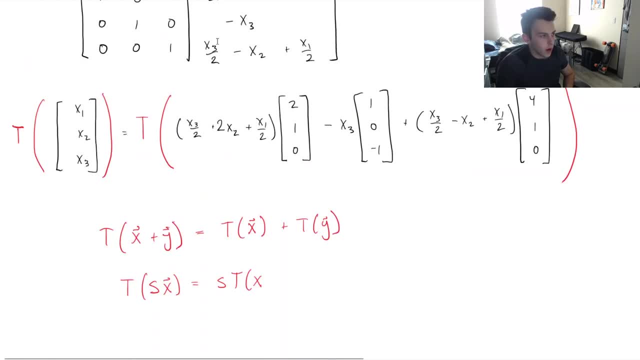 how we do have that three times Right. You've got this, this first vector multiplied by some scalar, and then we've got we're adding another vector multiplied by a scalar, and then we're adding another vector. 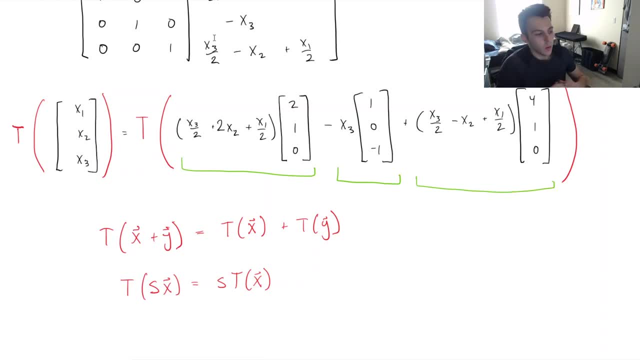 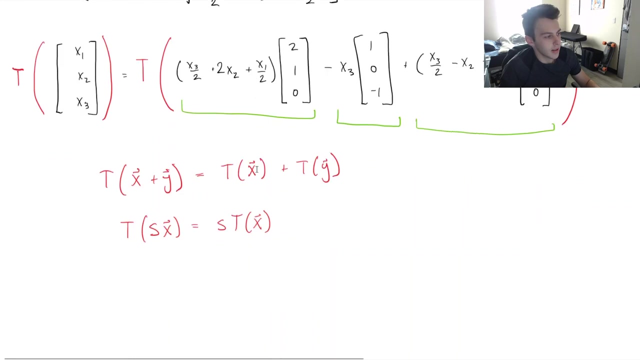 multiplied by a scalar. So what the key thing to to notice here is that linear transformations are conserved under linear combinations. So we can break this up. So let let's- let's simplify this a little bit. 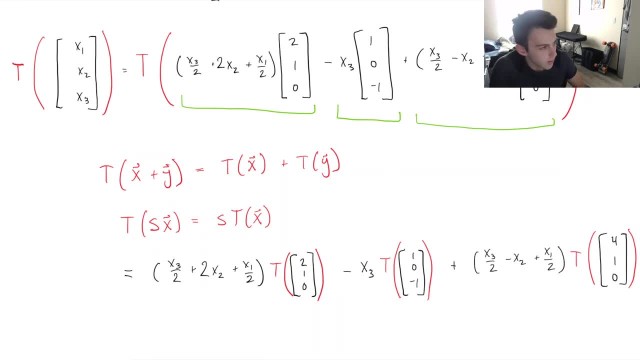 So what I've done here is I've broken up my transformations by the vectors and then all I did was pull out those constants. Right, So it's just applying that first law and then applying that second law. 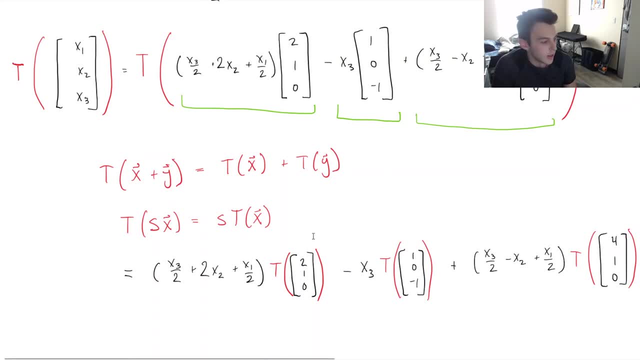 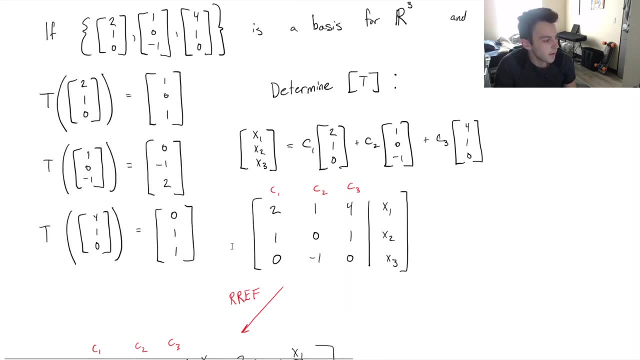 Right Back to back And what we know is that we actually know what these, these basis vectors, transform to. It tells us that in the question Right here. So let's, let's, substitute those values into. 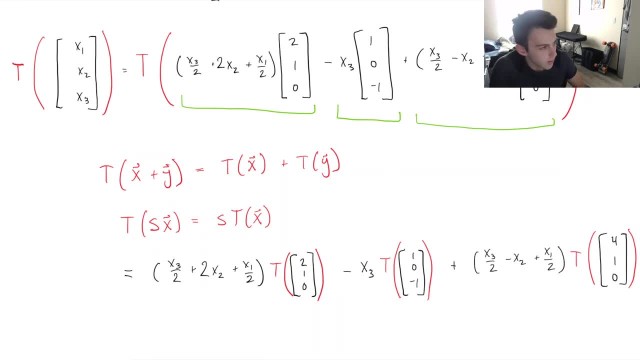 So what I've done here is I've broken up my transformations by the vectors and then all I did was pull out those constants. Right, So it's just applying that first law and then applying that second law. 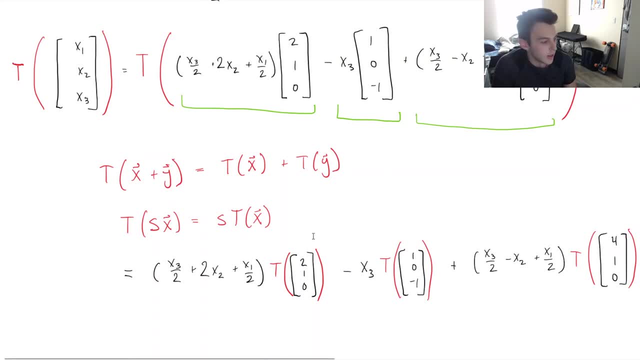 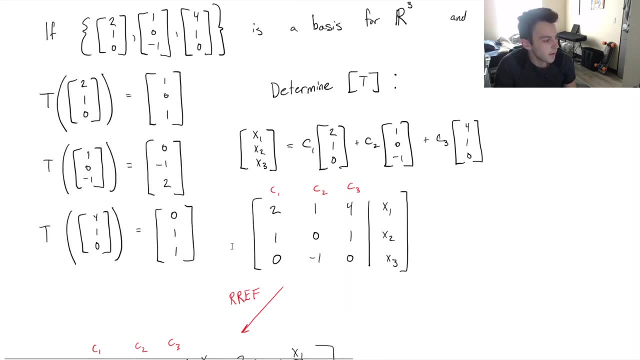 Right Back to back And what we know is that we actually know what these, these basis vectors, transform to. It tells us that in the question Right here. So let's, let's, substitute those values into. 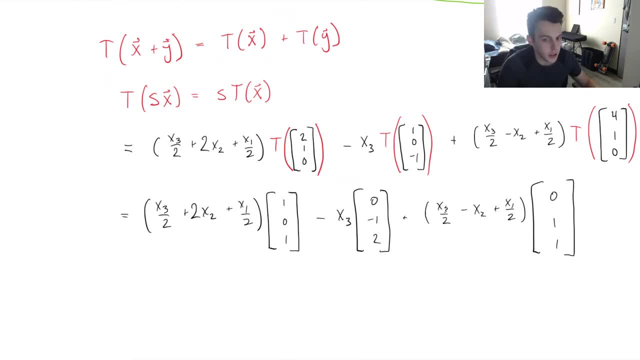 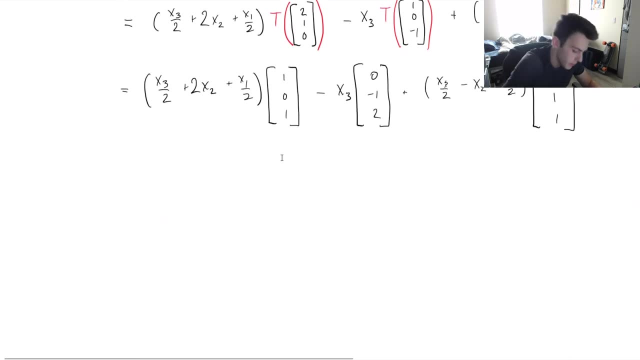 those transformed vectors, So I just I just rewrote them after substituting in what the question gives us. And now all we're doing is just adding vectors, Right, And we can reduce this or simplify this. 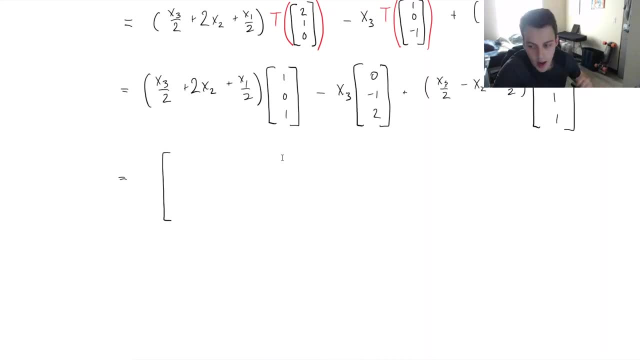 as much as we can, Right? So let's start with our x1 terms. Okay, So I've got in the first coordinate. I've got x1 multiplied by 0. So I've got. 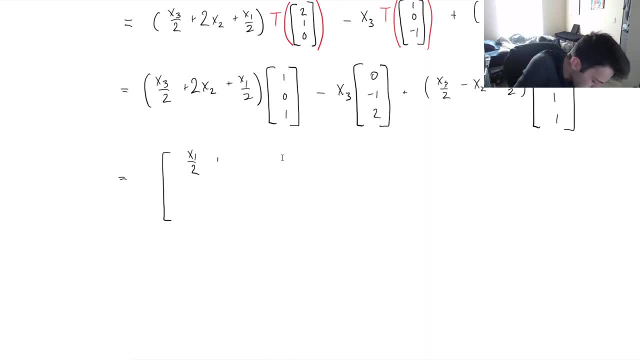 x1 over 2.. And then I've got 2 x2's And I've got x3, over 2.. That's our first coordinate, So our second, let's look. take a look at our second coordinate. 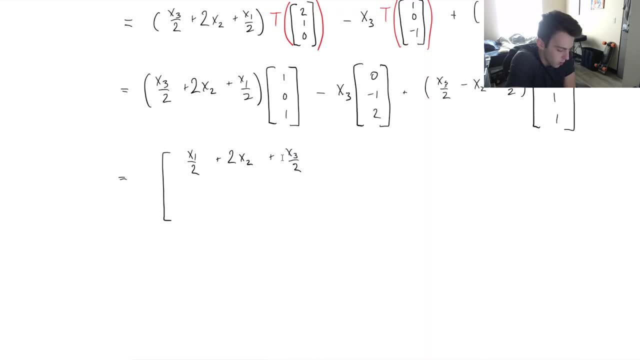 How many x1's? Well, the first vector, multiply, is multiplied by 0.. I've got an x3 in the second one And it looks like I've got an x1 over 2.. And I've got. 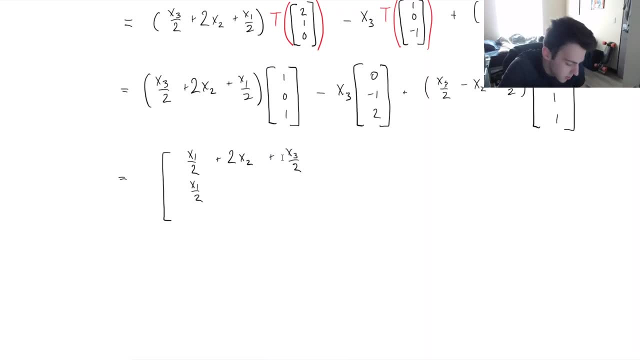 an x1 over 2.. And let's take a look at our x2's. It looks like I've just got a a minus x2 here And then I've got a positive x3.. And 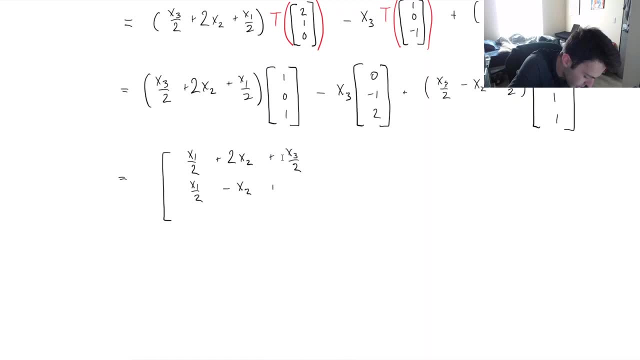 then I'm adding another x3, over 2.. So that's gonna be 3 over 2, x3. Great. Lastly, I've got, okay, my x1's I've got from my first. 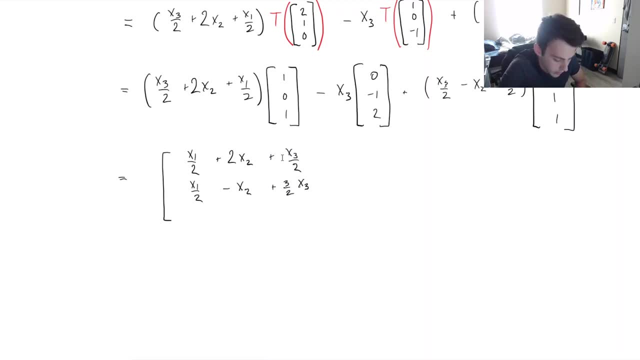 my first vector: I've got an x1 over 2.. My last vector: I've got, I've got another x1 over 2.. So adding them together, I'll get a single x1.. And then my x2's. 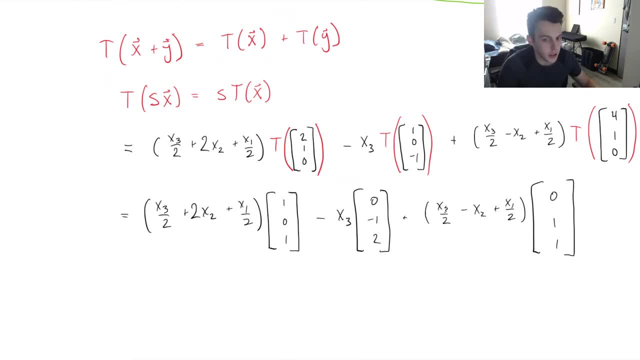 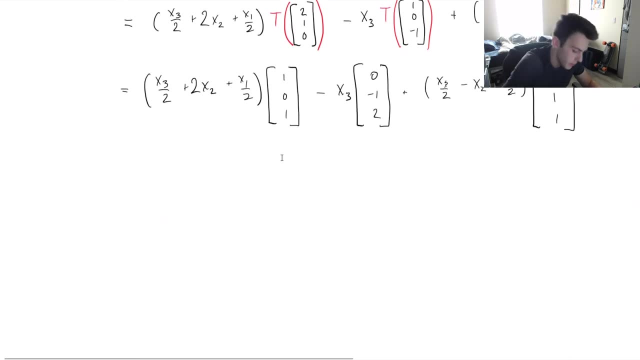 those transformed vectors, So I just I just rewrote them after substituting in what the question gives us. And now all we're doing is just adding vectors, Right, And we can reduce this or simplify this. 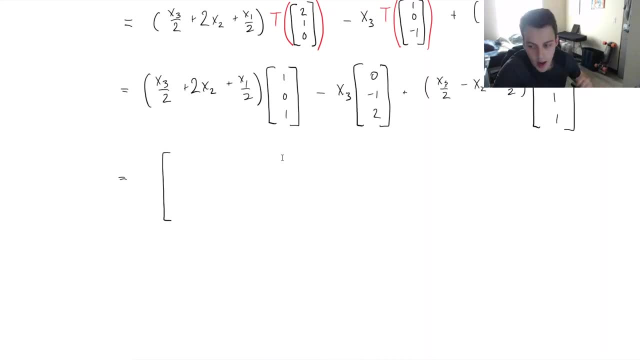 as much as we can, Right? So let's start with our x1 terms. Okay, So I've got in the first coordinate. I've got x1 multiplied by 0. So I've got. 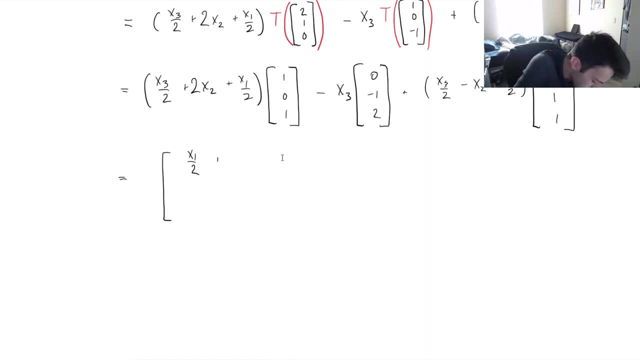 x1 over 2.. Then I've got 2 x2's And I've got x3, over 2.. That's our first coordinate, So our second, let's look. take a look at our second coordinate. 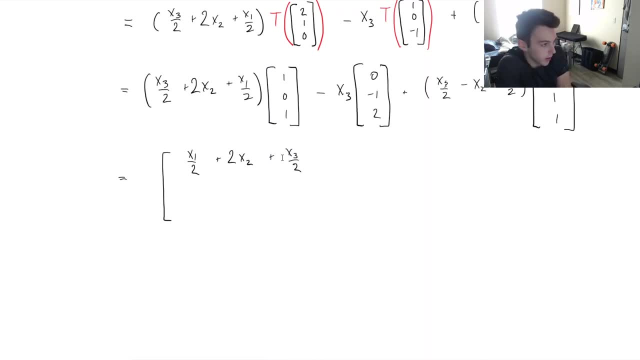 How many x1's? Well, the first vector, multiply, is multiplied by 0.. I've got an x3 in the second one And it looks like I've got an x1 over 2.. And I've got. 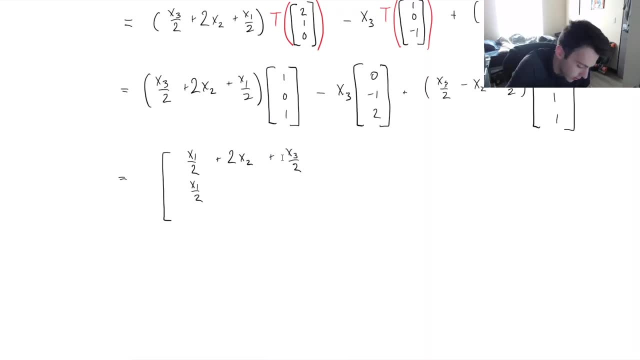 let's take a look at our x2's. It looks like I've just got a a minus x2 here, And then I've got a positive x3.. And then I'm adding another x3,. 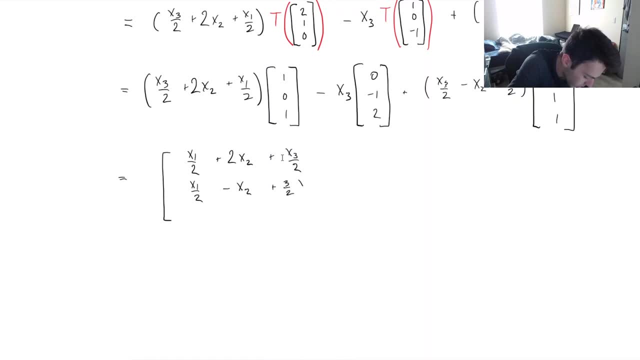 over 2.. So that's gonna be 3 over 2, x3.. Great. Lastly, I've got. okay, my x1's I've got from my first, my first vector, I've got. 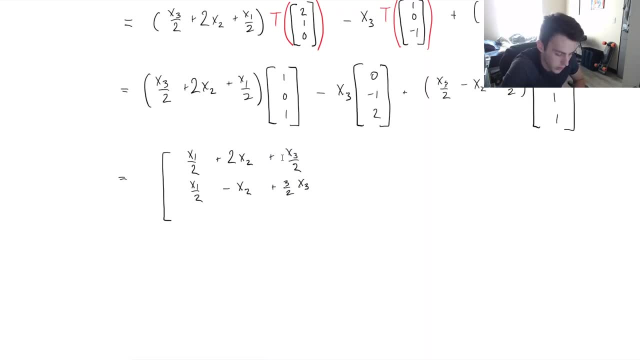 an x1 over 2.. My last vector. I've got another x1 over 2.. So adding them together I'll get a single x1. And then my x2's. I've got 2x2 from the first vector. 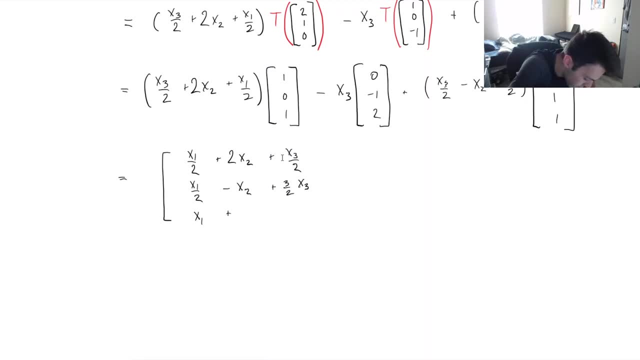 And then I'm subtracting an x2.. So that's a positive x2.. And then, lastly, I've got x3 over 2, from the first one, And then I'm subtracting. 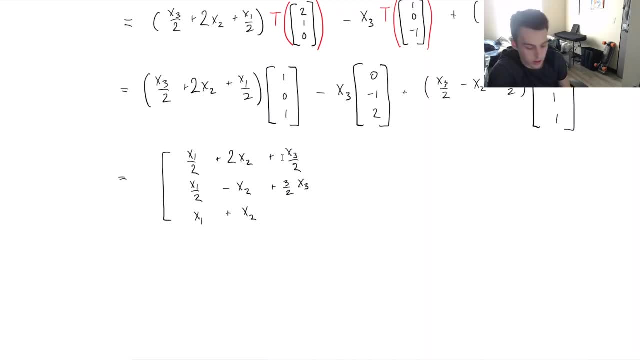 2x3's, but then I'm adding another x3.. So this minus x3.. If I've done that right, Awesome, Okay. So now you might notice that I've got it looks very much.